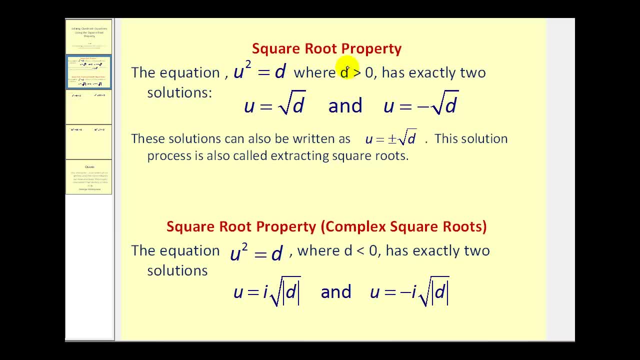 which states that the equation u squared equals d where d is greater than zero, has exactly two solutions, where u is equal to the square root of d and u is equal to the negative square root of d, And sometimes this is written as u equals plus or minus the square root of d. 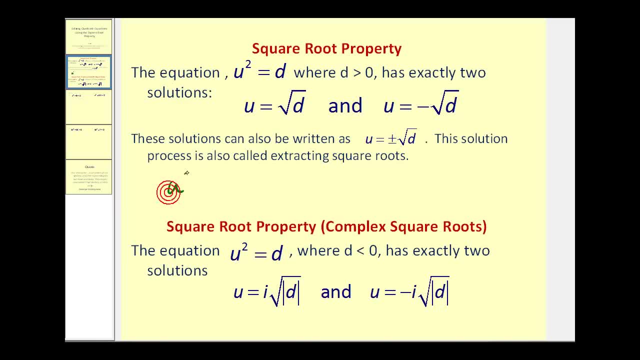 So what this is trying to tell us is: if we had u squared equals thirty-six, then u would equal positive square root of thirty-six, which is six, and u would also equal negative square root of thirty-six, which is equal to negative six. 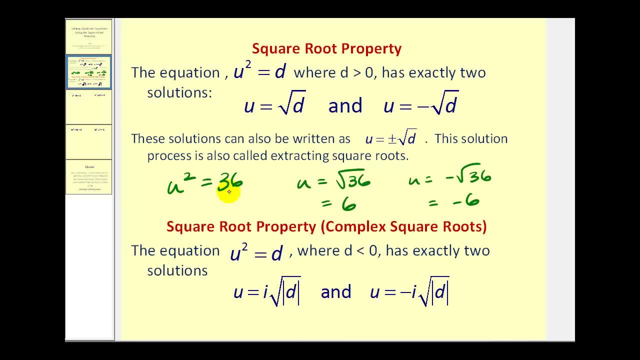 Remember, if we square negative six, we still get positive thirty-six, So we'll have a positive and a negative solution And notice that if d is negative or less than zero, there are still two solutions. It's just now that we have imaginary solutions. 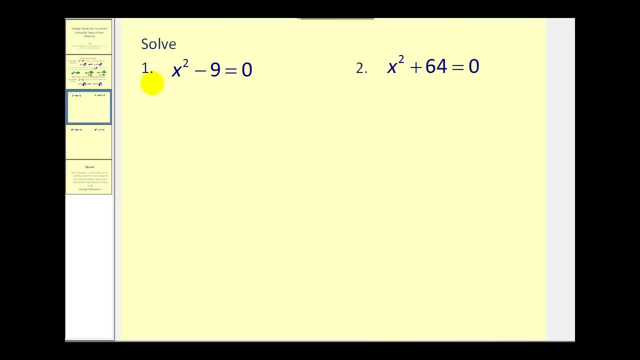 Let's go ahead and take a look at some examples. So, even though number one is factorable as a difference of squares, we're going to go ahead and solve this using the square root property. So let's go ahead and add nine to both sides. 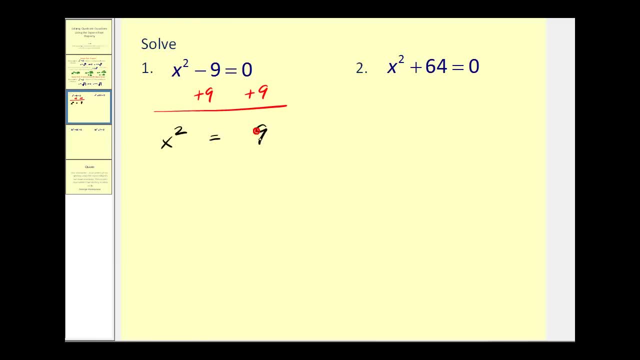 So we'll have x squared equals nine. Now, if we have x squared and we want x, we can take the square root of both. We can take the square root of both sides of the equation, as long as we remember to include a plus or minus to obtain the two solutions. 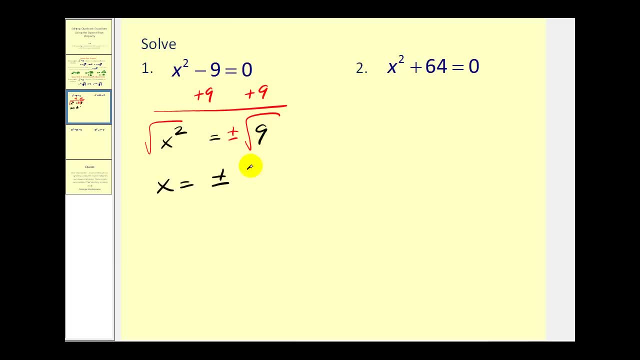 So we have: x equals plus or minus the square root of nine, which is three, And if we wanted to, we can list this as x equals three and x equals negative three, But often you'll see the answer written in this form to represent both solutions. 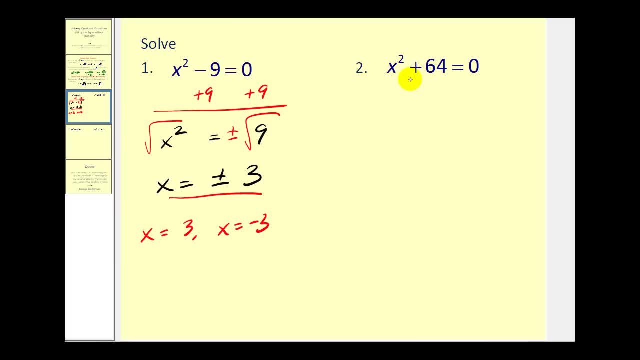 Okay, and number two: notice: this is not factorable because we have a sum of squares, but we can use the square root property to solve this. So we'll subtract 64 on both sides. So we have x squared equals negative 64.. 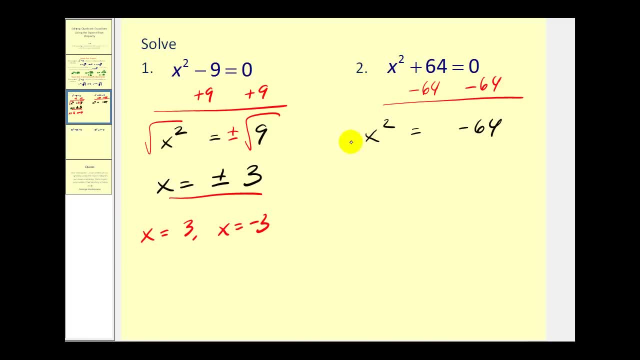 Now, to get x from x squared, we'll take the square root of both sides And again plus or minus. So we'll have: x equals plus or minus the square root of negative one times 64.. Well, the square root of negative one would be i. 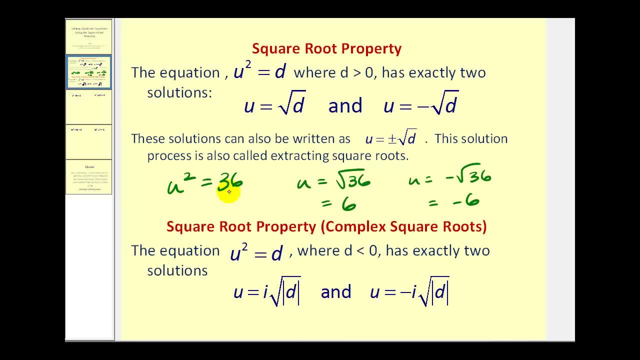 Remember, if we square negative six, we still get positive thirty-six, So we'll have a positive and a negative solution And notice that if d is negative or less than zero, there are still two solutions. It's just now that we have imaginary solutions. 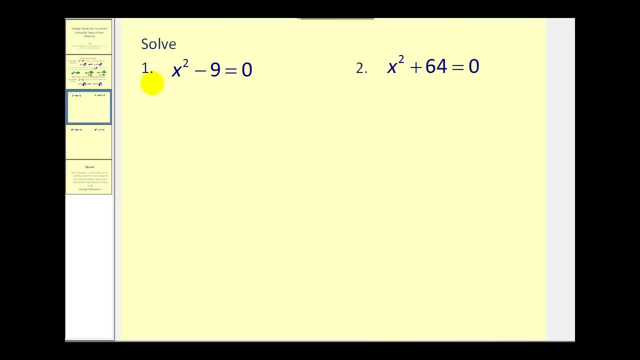 Let's go ahead and take a look at some examples. So, even though number one is factorable as a difference of squares, we're going to go ahead and solve this using the square root property. So let's go ahead and add nine to both sides. 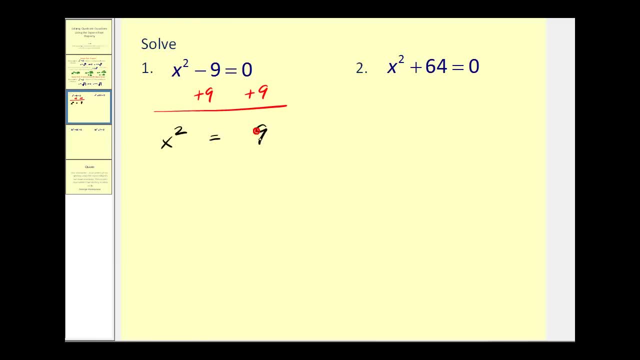 So we'll have x squared equals nine. Now, if we have x squared and we want x, we can take the square root of both. We can take the square root of both sides of the equation, as long as we remember to include a plus or minus to obtain the two solutions. 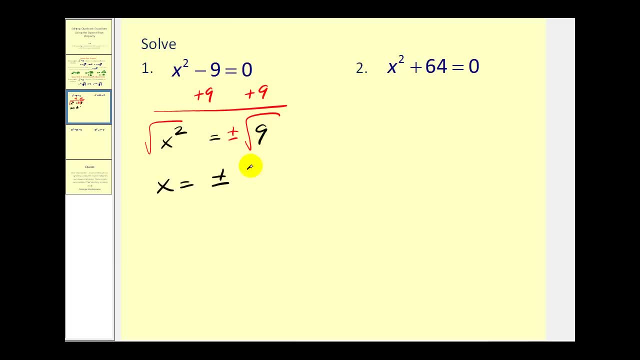 So we have: x equals plus or minus the square root of nine, which is three, And if we wanted to, we can list this as x equals three and x equals negative three, But often you'll see the answer written in this form to represent both solutions. 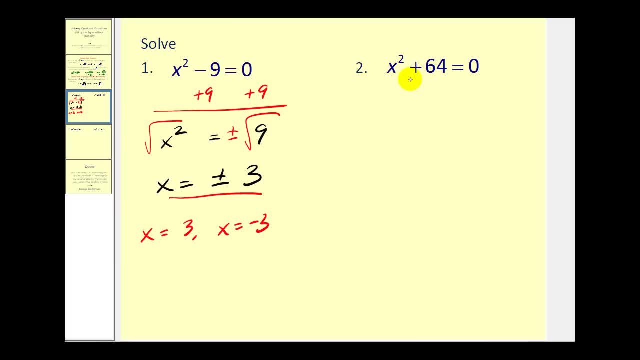 Okay, on number two notice: this is not factorable because we have a sum of squares, But we can use the square root property to solve this. So we'll subtract sixty-four on both sides. So we have x squared equals negative sixty-four. 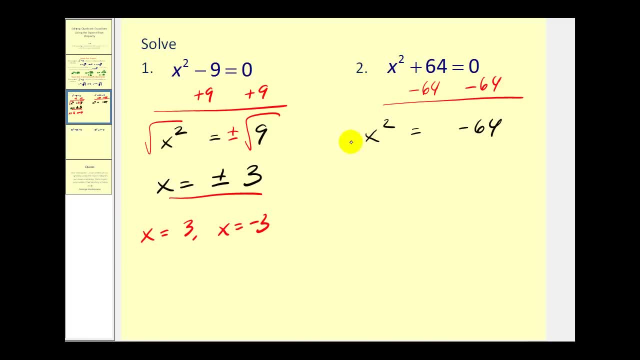 Now, to get x from x squared, we'll take the square root of both sides And again plus or minus. So we'll have: x equals plus or minus the square root of negative one times sixty-four. Well, the square root of negative one would be i: 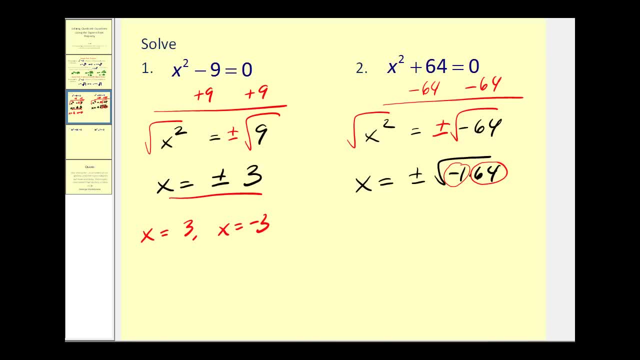 The square root of sixty-four would be eight. So we have: x equals plus or minus eight i, Or x equals eight i and x equals negative eight i. Let's go ahead and take a look at a couple more of these. Okay, on number three, again we're trying to isolate the x squared. 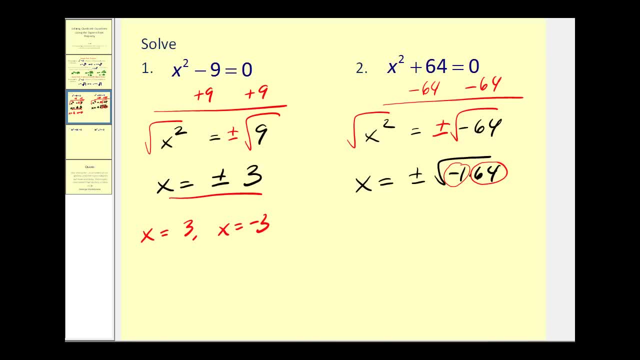 The square root of 64 would be eight. So we have x equals plus or minus eight i, Or x equals eight i and x equals negative eight i. Let's go ahead and take a look at a couple more of these. Okay, and number three. again, we're trying to isolate the x squared. 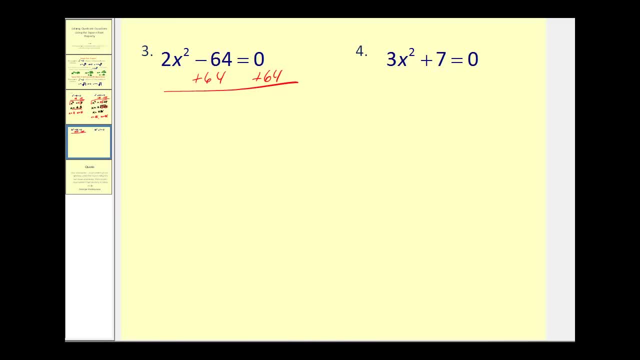 so we'll add 64 to both sides. So we have two x squared equals 64.. Now, in order to isolate the x squared, we still have to divide by two in this problem. So we'll have x squared equals 32.. And now we can square root both sides of the equation. 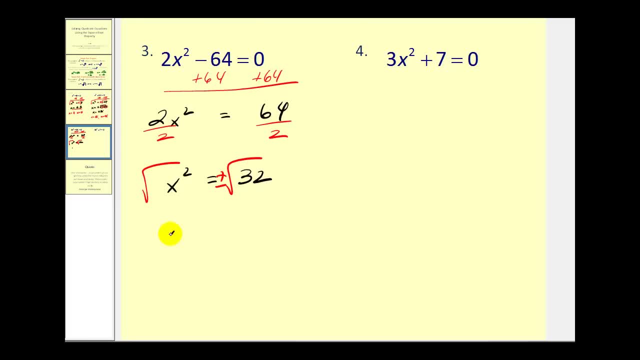 Plus or minus there. So we have x equals plus or minus the square root of 32.. But 32 is equal to 16 times two. 16 is a perfect square. So we have x equals plus or minus four, square root two. 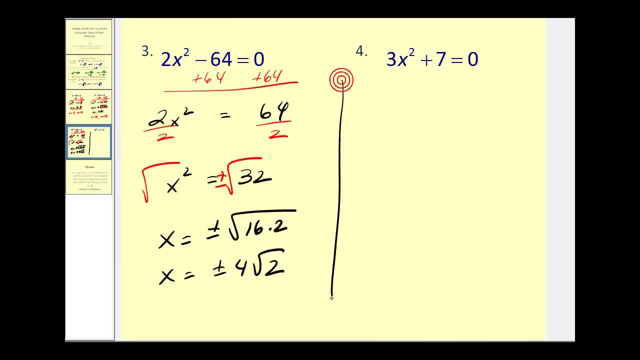 And let's take a look at one more Again. we need to isolate the x squared, So we'll go ahead and subtract seven on both sides. So we have three. x squared equals negative seven. Now we need to divide by three, So we have x squared equals negative seven thirds. 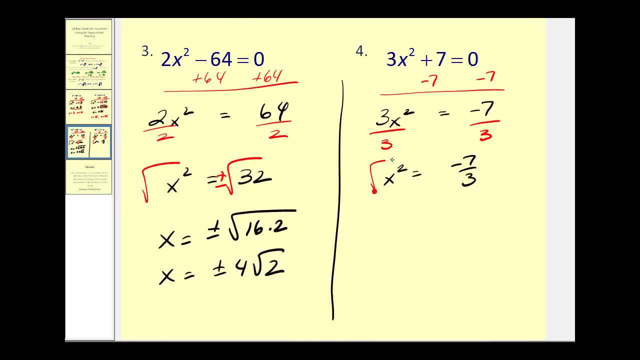 Now we'll square root both sides of the equation And there's our two solutions. So we have x equals plus or minus. Remember we can't leave a fraction underneath the square root, So we could rewrite this as: square root negative seven over square root three. 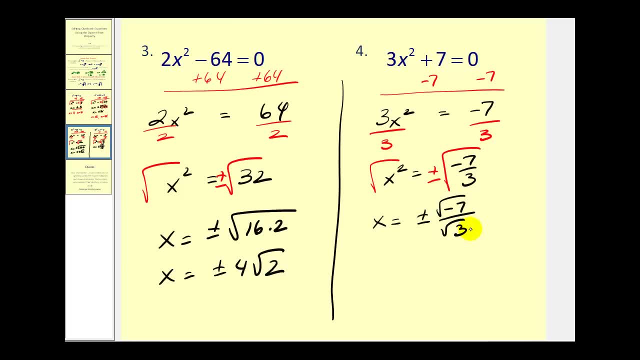 But now we can't have a square root in our denominator. So we'll multiply denominator and the numerator by square root three. So we'll have x equals plus or minus square root of. Well, this would be negative 21, or negative one times 21.. 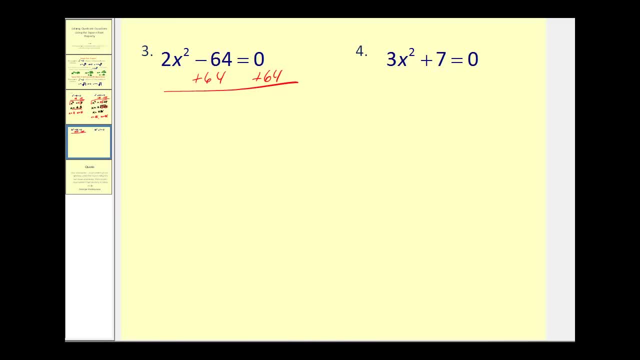 So we'll add sixty-four to both sides. So we have two x squared equals sixty-four. Now, in order to isolate the x squared, we still have to divide by two in this problem. So we'll have x squared equals thirty-two. And now we can square root both sides of the equation. 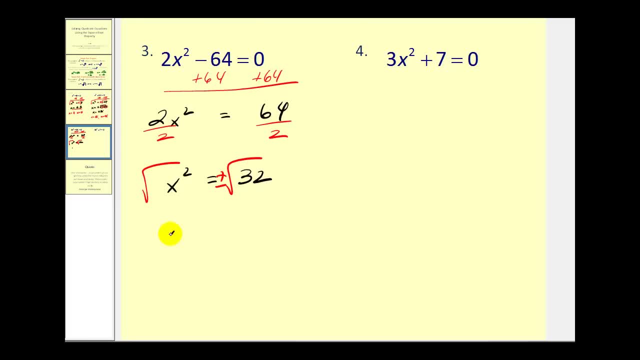 Plus or minus there. So we have x equals plus or minus the square root of thirty-two. But thirty-two is equal to sixteen times two. Sixteen is the perfect square, So we have x equals plus or minus four square root of two. 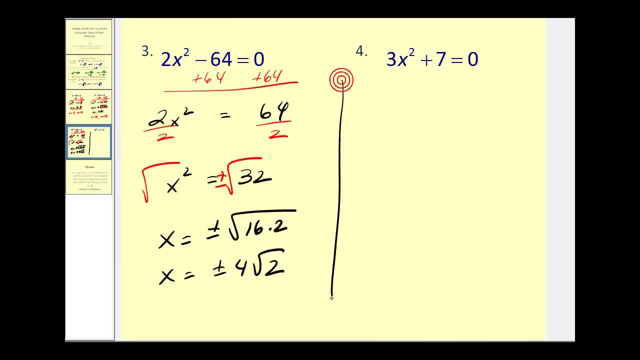 And let's take a look at one more Again. we need to isolate the x squared, So we'll go ahead and subtract seven on both sides. So we have three. x squared equals negative seven. Now we need to divide by three, So we have x squared equals negative seven thirds. 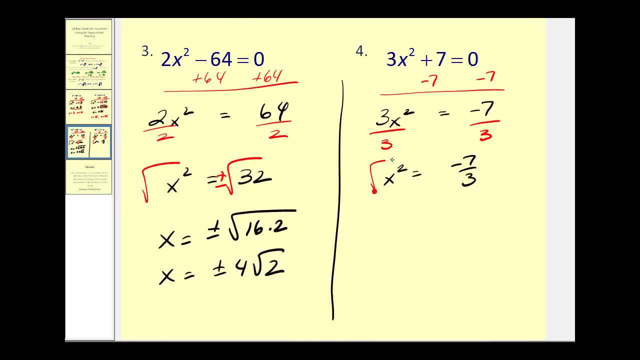 Now we'll square root both sides of the equation And there's our two solutions. So we have x equals plus or minus. Remember we can't leave a fraction underneath the square root, So we could rewrite that It says square root negative seven over square root three. 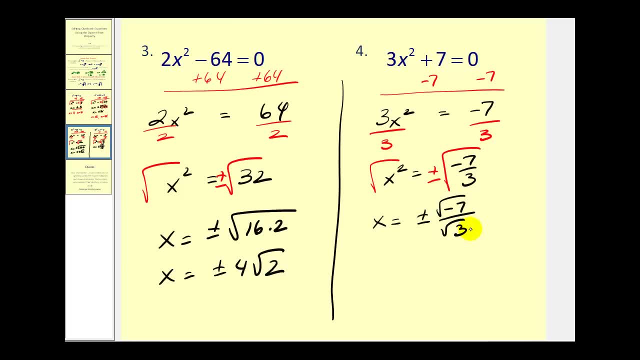 But now we can't have a square root in our denominator, So we'll multiply the denominator and the numerator by square root three. So we'll have x equals plus or minus square root of. Well, this would be negative twenty-one, or negative one times twenty-one. 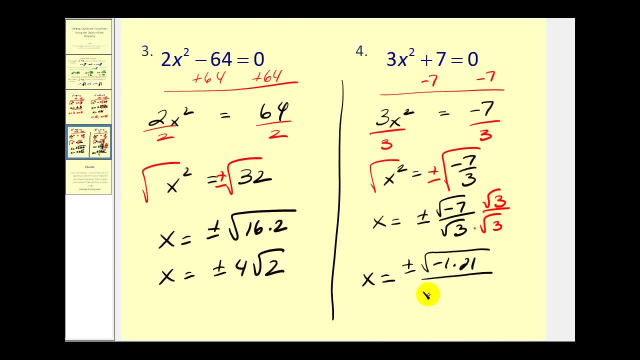 All over the square root of three times three. So we're going to have plus or minus i square root twenty-one all over three. Again, notice we have a positive and a negative solution. Okay, I hope you found this video helpful. Thank you for watching. I'll see you in the next video. Totally Thanks for watching, Bye, bye. Transcript provided by.